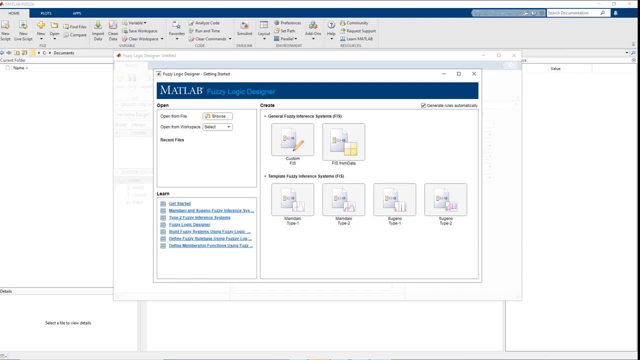 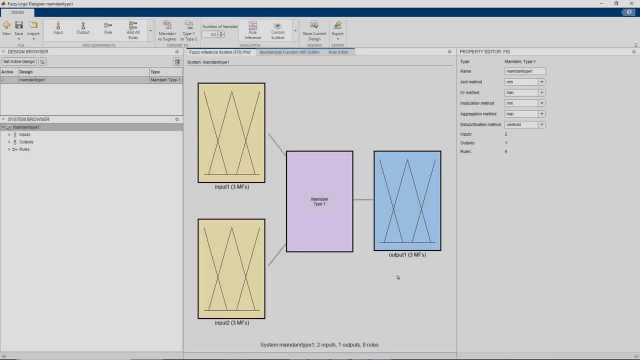 For this example, we will use the Mamdani Type 1 template to get started. The template creates a standard fuzzy system, as seen in the fuzzy inference plot, and loads the default set of membership functions. Let us name the inputs and the output. 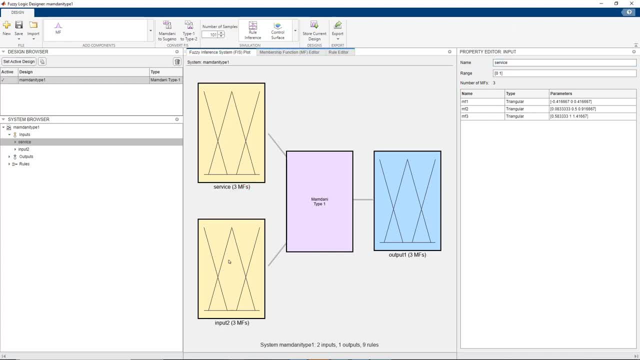 Now that we have the structure decided, The next steps are to define the membership function. To define or add membership functions to inputs and outputs, you can click on the corresponding entry in the system browser and make the required changes in the property editor. For this example, for the first input, which is service, we shall use three Gaussian membership functions to model poor, good and excellent service and enter the corresponding values for the parameters. 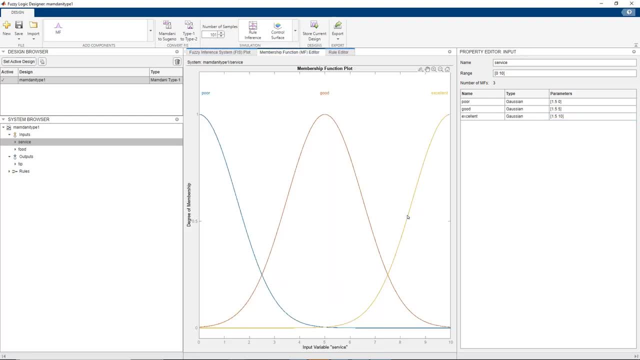 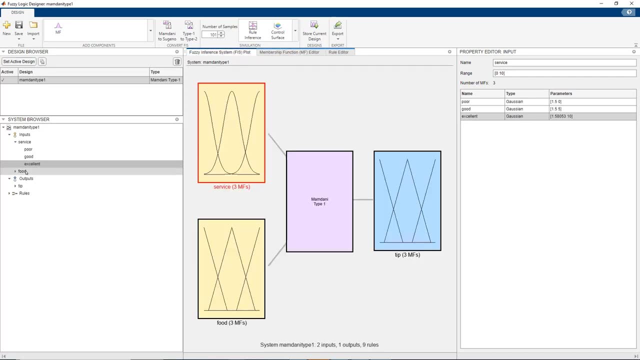 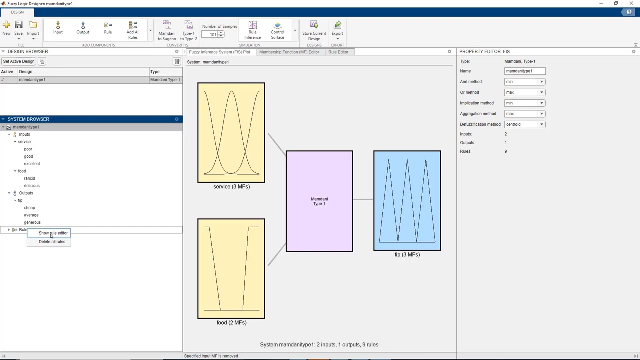 These parameters can also be modified graphically Using the membership function plot. we will repeat similar steps for the other inputs, food and output tip. The next step is to map the inputs to output using rules. To do this, right click on rules in the system browser and click on Show Rule Editor. 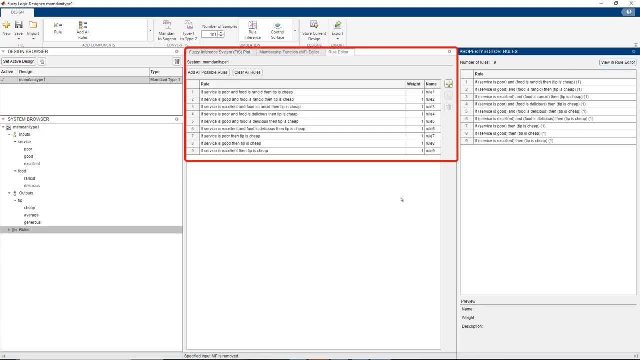 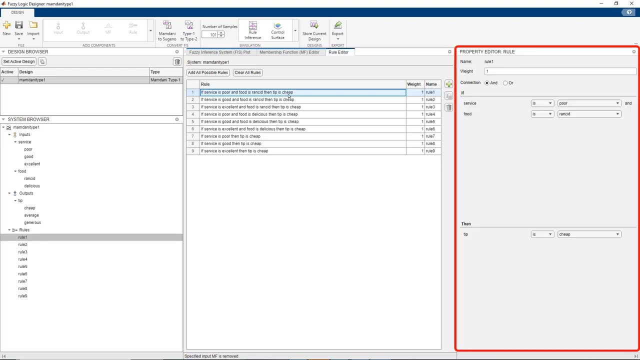 You can use the rule editor to add, copy or delete rules and manage all rules of your system, and then use the property editor tab associated with it to make changes to individual rules. The rule editor also provides the option to automatically populate all possible rules. 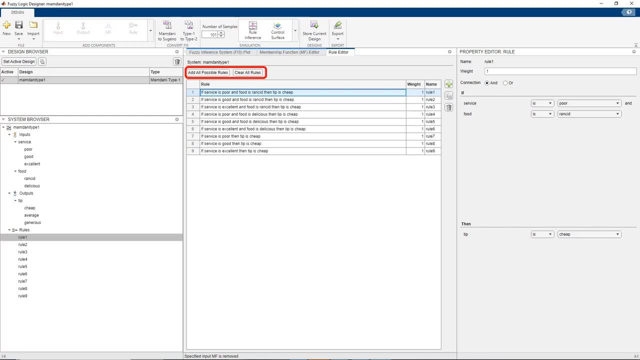 by including all combination of inputs and its membership functions For this example. we would like to create three simple rules to design the logic. Let us implement the rules. The first rule is: if service is poor or food is rancid, then the tip is cheap. 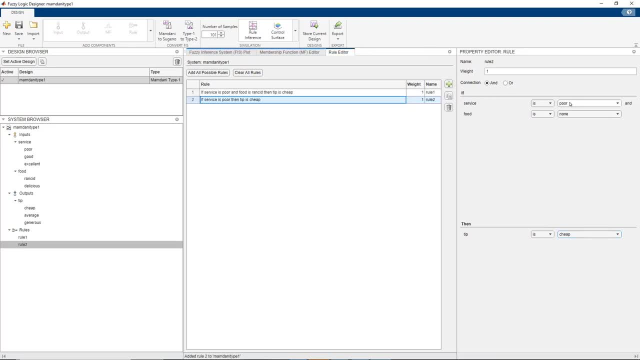 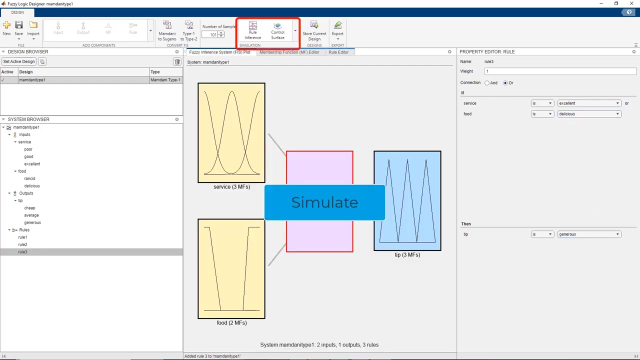 Second: if service is good, the tip is average. In this case the second input, food, has no implications here, So we can enter that as none. And the last rule: if service is excellent or food is delicious, the tip is generous. We can now go ahead and simulate our system. 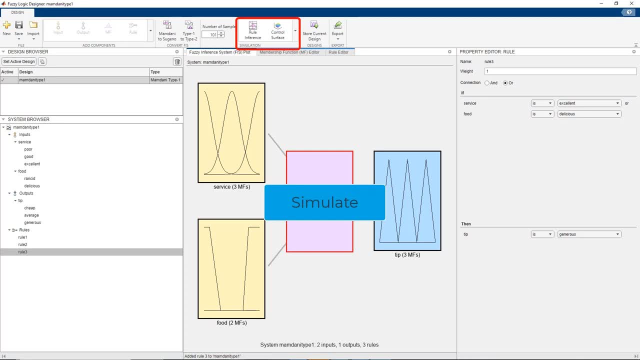 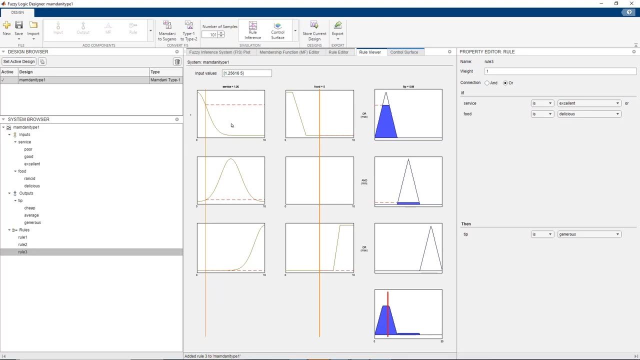 To do so, you can use the rule inference and control surface to evaluate your design. Click on rule inference to open the rule viewer. Here you can make changes to your inputs by using a slider to model different scenarios and evaluate how your fuzzy system respond.